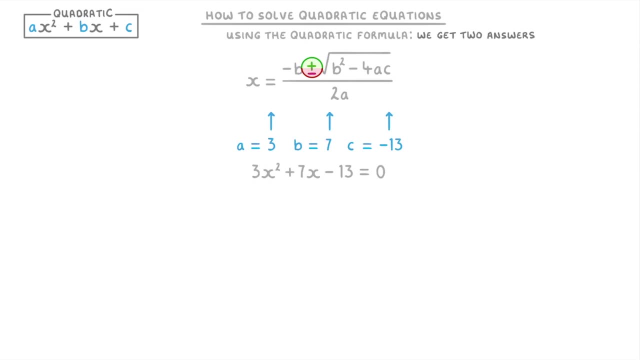 plug. So if we start with the plus sign one, we'd get x equals minus 7, because, remember, b is 7, plus the square root of 7, squared minus 4, times 3 for the a and times negative 13. 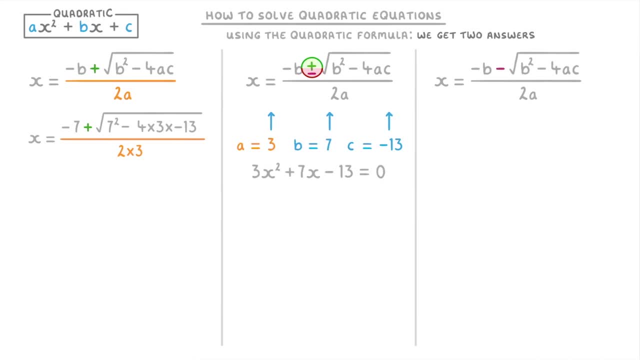 for the c All divided by 2 times 3.. So we've got x equals minus 7, because, remember, b is 7, plus the square root of 7 squared times 3.. And then for the minus version, we get exactly the same thing, except we're. 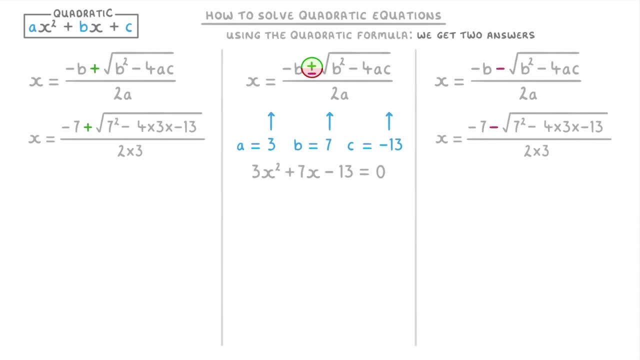 subtracting the big square root. If they ask for the solution to a certain number of decimal places, like give your answer to two decimal places, then you can just plug the whole thing straight into your calculator, which for this one on the left would be 1.22, and for the 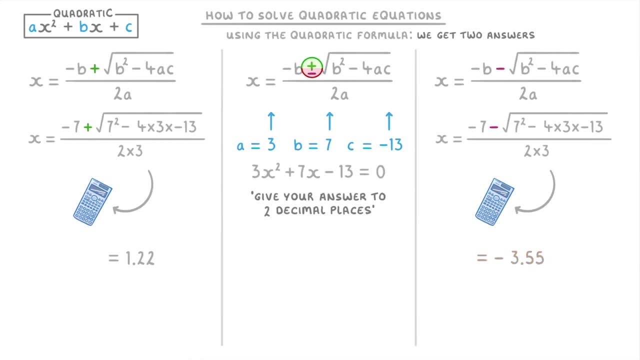 one on the right would be negative 3.55.. But you do need to be careful because if you do, it's really easy to make a mistake. The most common problem is with this minus sign inside the square root, so it's always best to stick these four ac bits in a bracket. 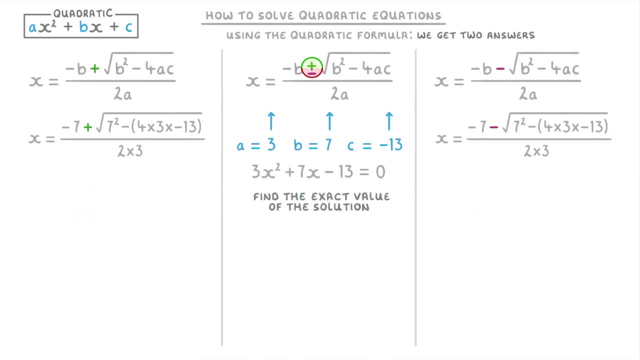 Now sometimes you might be asked instead to find the exact value of the solution, which means that you can't round it to a certain number of decimal places or significant figures. Instead, you have to just simplify it down as much as you can. If we try this for our minus version on the right, the minus 7 can't be simplified. But 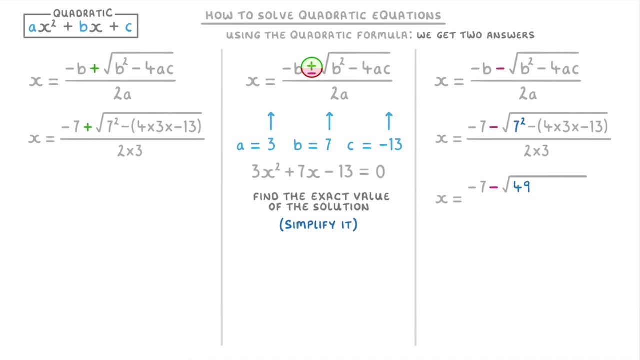 inside the square root we can change the 7 squared to 49, and the takeaway 4 times 3, times negative 13, to minus negative 156. And then on the bottom we can simplify the 2 times 3 to just divide by 6.. Then if we do the 49 minus negative 156, the two negatives 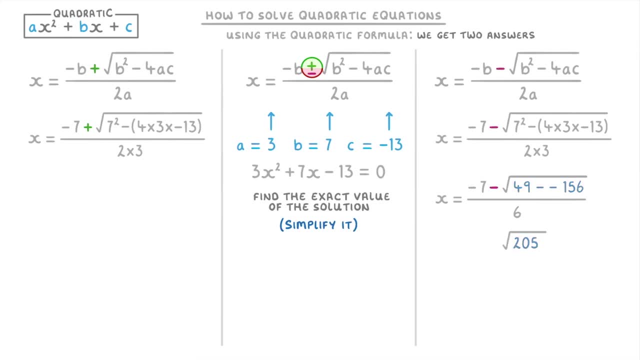 plus and we get positive 205 in the square root, while the rest of the answer stays the same. Sometimes you might be able to simplify down the root, but in this case we can't. so this is the most simple it can go, and we'd leave our answer like this.